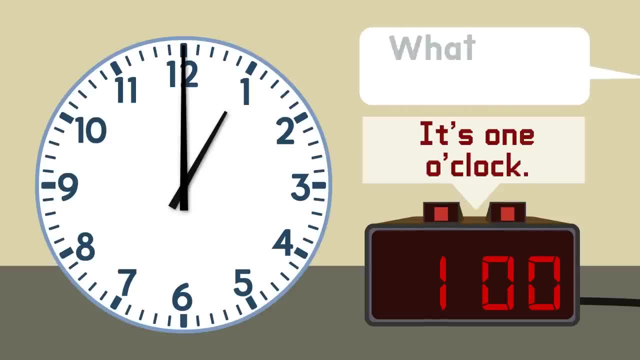 What time is it? It's 1 o'clock. What time is it? It's 1 o'clock. It's 1 o'clock. If the big hand's on the 12,, well then you'll know. If the big hand's on the 3,, well then you'll know. 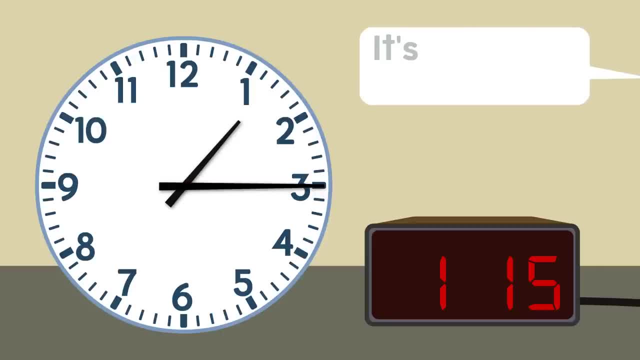 A quarter hour has passed, Let's go. It's a quarter after 1.. It's 1.15.. It's a quarter after 1.. It's 1.15.. If the big hand's on the 6,, well then you'll know. 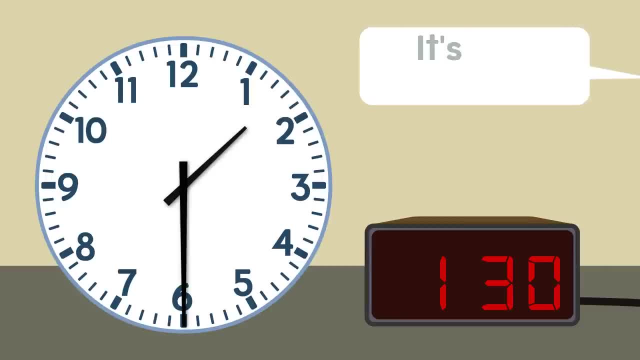 A half hour has passed. Let's go. It's half past 1.. It's 1.30.. It's half past 1.. It's 1.30.. It's 1.30.. If the big hand's on the 9,, well then you'll know. 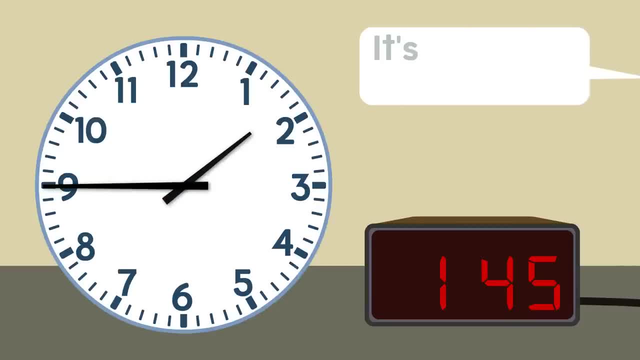 There's been 45 minutes and there's 15 to go. It's a quarter to 2.. It's 1.45.. It's a quarter to 2.. It's 1.45.. Look over, here We've got an analog clock. 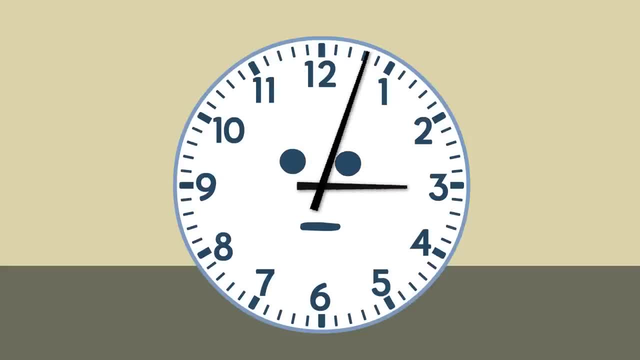 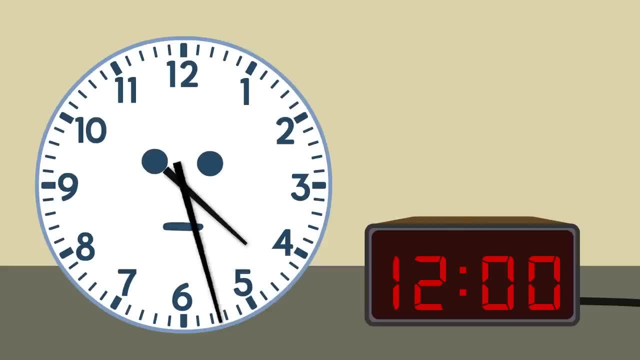 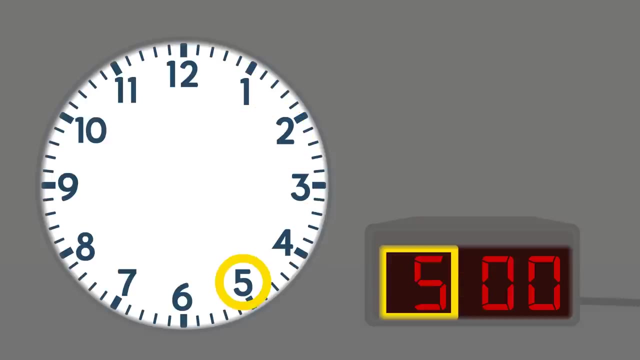 It has hands that go round and do not stop. And look right. here We've got a digital clock with more numbers And it can talk. I am still 8 o'clock. These numbers here go from 1 to 12 and then they start all over at number 1 again. 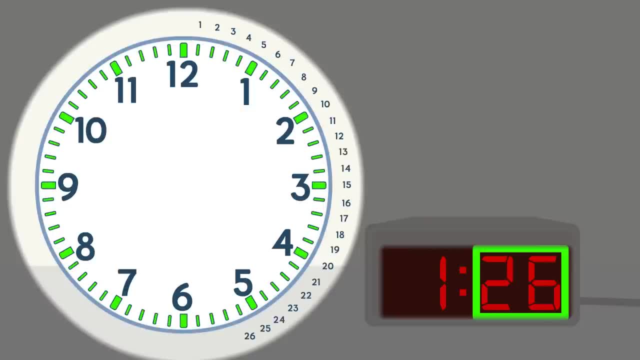 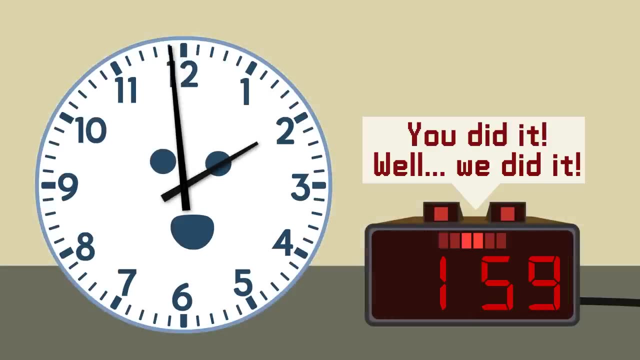 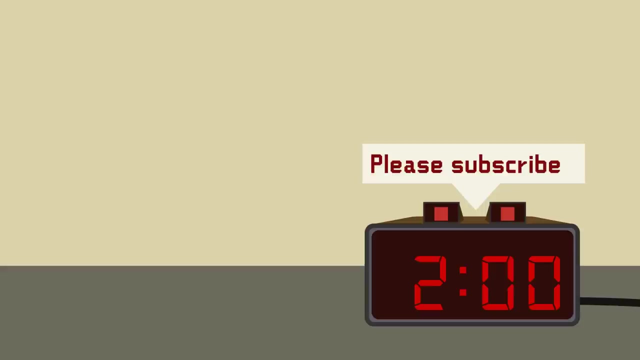 And these numbers go from 0 to 60. That's how to tell time. Thanks for staying with me. You did it Well. we did it together, You and I. Teamwork, Teamwork.